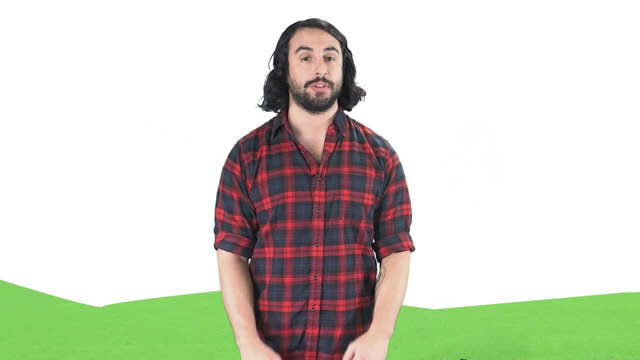 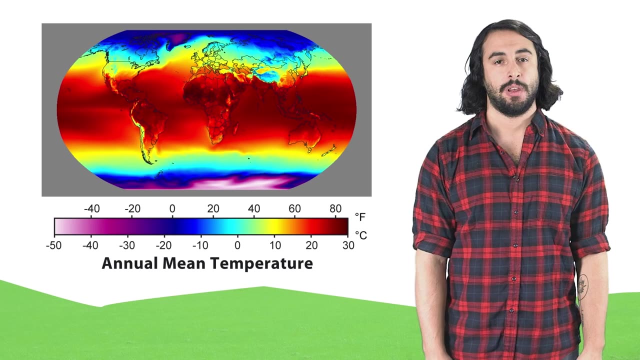 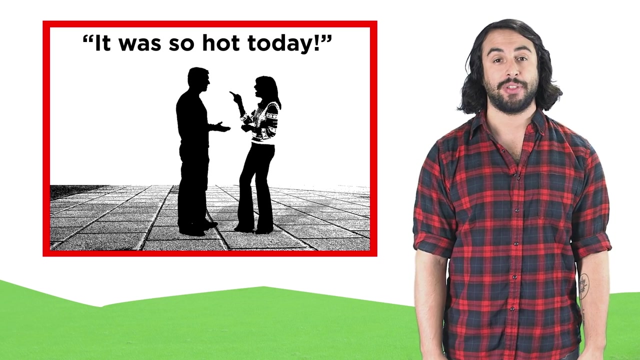 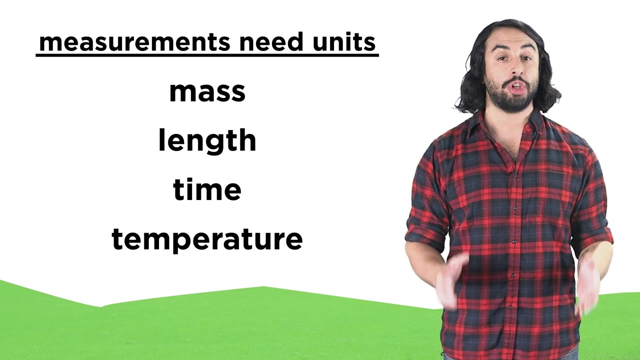 Hey, it's Professor Dave, let's learn how to do temperature conversions. Temperature is a big part of the human experience. If you want to make small talk in public, just bring up the temperature that day and you're good to go. But just like mass, length and time, we can use different units to measure temperature. 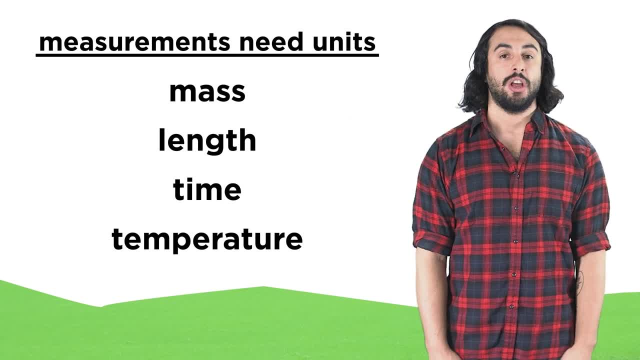 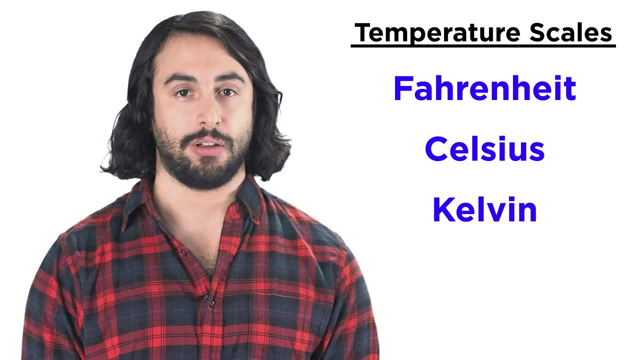 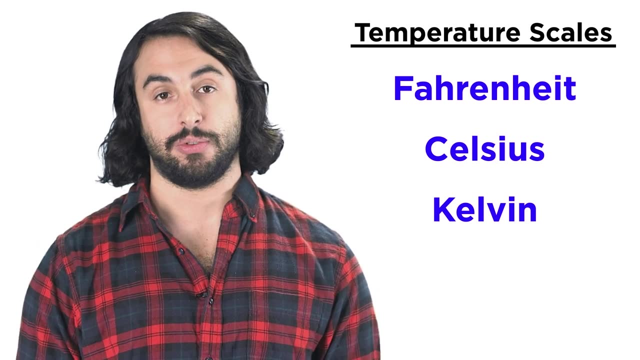 And we need to be able to convert between these units just as we would with any other set of units. Most people are familiar with just one temperature scale, which will depend on where they live in the world, But there are three that are commonly used, and these are Fahrenheit, Celsius and Kelvin. 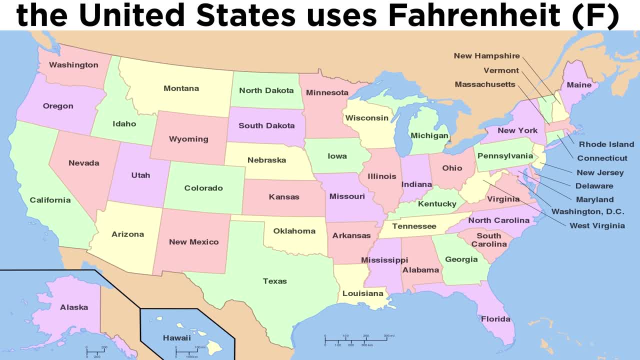 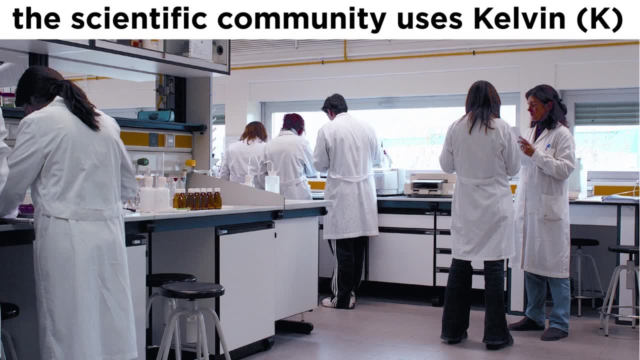 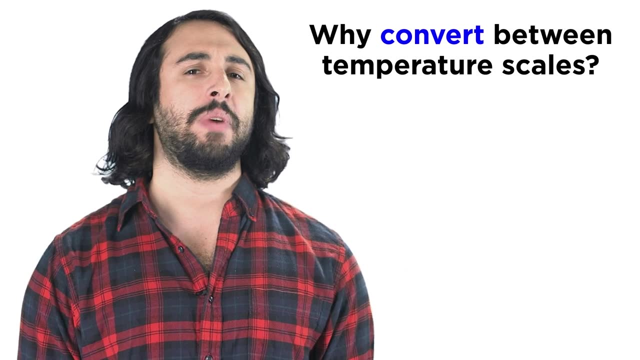 Fahrenheit is used only in the United States and a handful of US territories. The rest of the world uses Celsius and the scientific community will typically use Kelvin when doing calculations. as this is the SI unit for temperature, Why would we need to convert between temperature units? 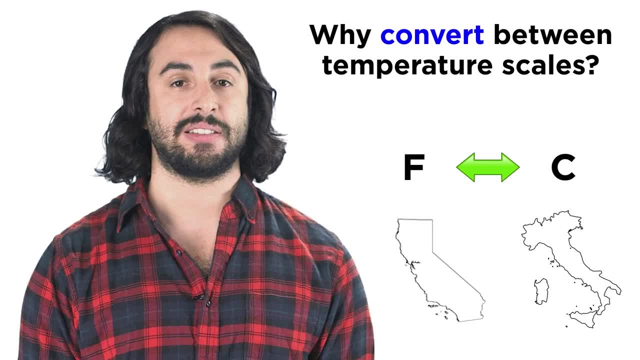 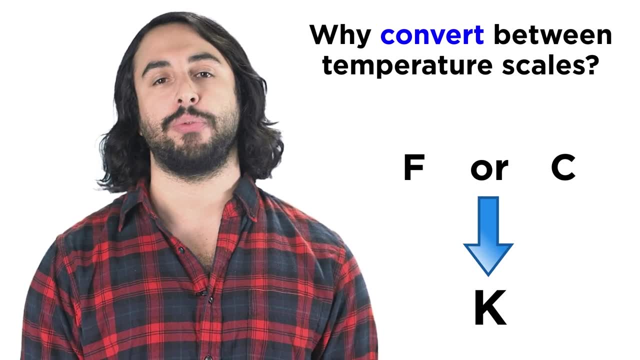 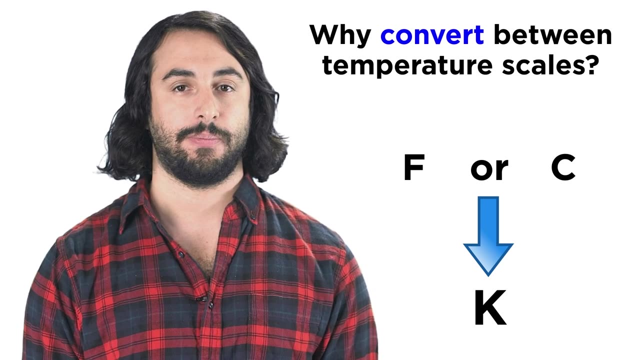 Well, we could convert between Fahrenheit and Celsius to figure out whether it was hotter in California or Italy on any given day, Or we might need to convert a temperature from one of those scales into Kelvin in order to do scientific calculations. So let's learn about the equations that will allow us to make these conversions. 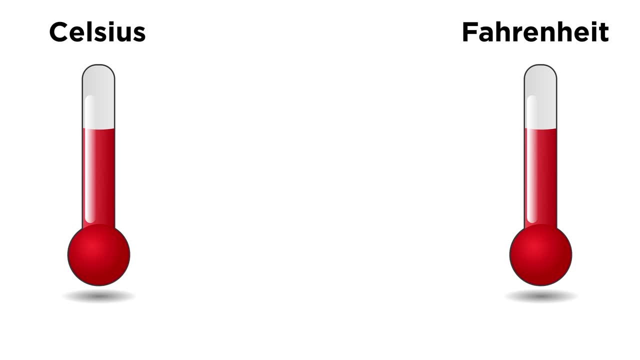 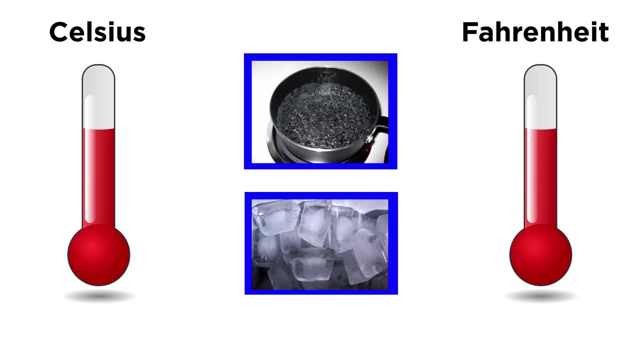 In order to put these temperature scales into context, we must understand the reference values that each scale uses. Both Fahrenheit and Celsius are defined using the freezing point and boiling point of water. Celsius sets the freezing point of pure water at zero and the boiling point at 100, splitting 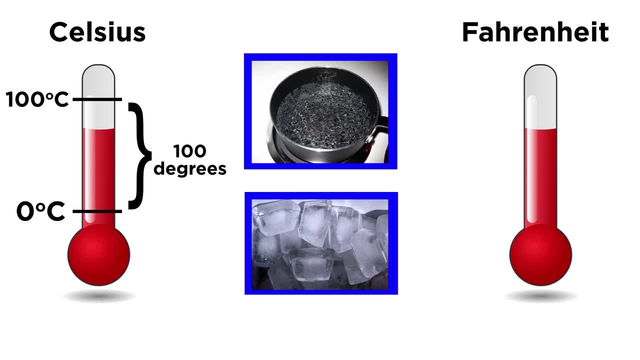 up the space between into 100 equal parts, called degrees. Fahrenheit, a little less intuitively, sets zero as the freezing point of brine, which is a salt water solution. That puts the freezing point of pure water at 32, and the boiling point at 212, splitting 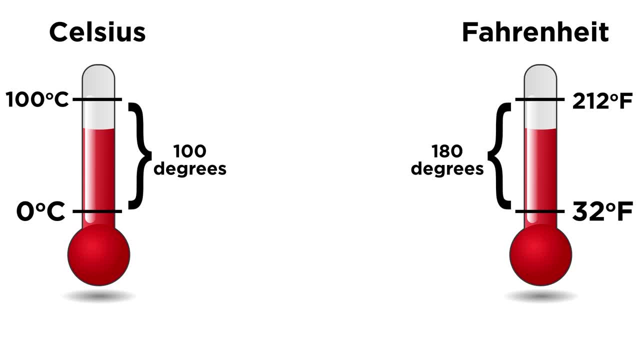 up the space between them into 180 degrees. So to understand how to convert between these, we must realize that Fahrenheit climbs 180 degrees In the same space that Celsius climbs 180 degrees In the same space that Celsius climbs 100, which requires that Fahrenheit temperatures. 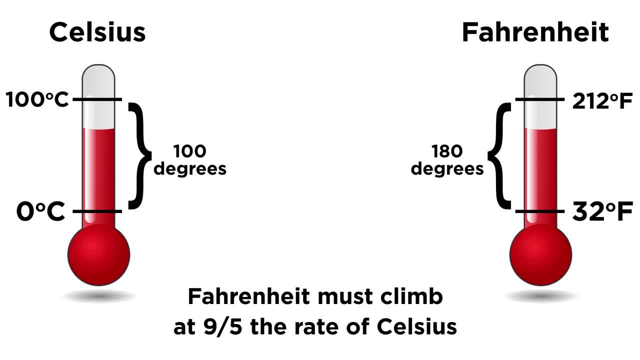 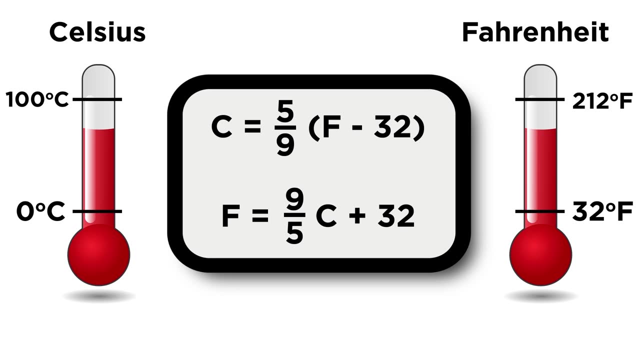 climb at nine-fifths the rate of Celsius temperatures, But there is also a 32 degree discrepancy in where these segments begin, and this also has to be accounted for. That means that these will be the two equations we can use when converting in one direction. 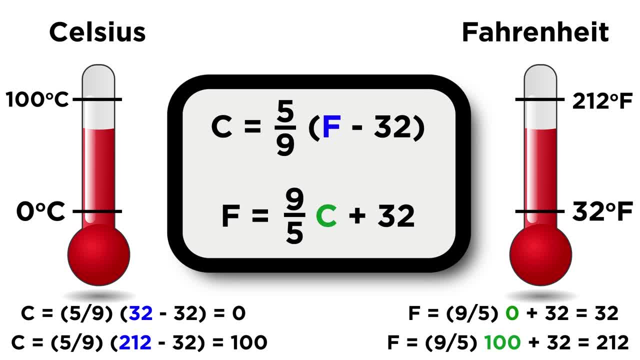 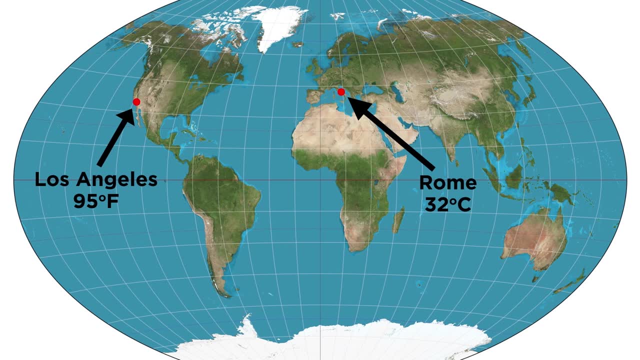 or the other. Let's test them by plugging in the freezing and boiling points of water to ensure that we get valid results, And we can see that each conversion goes precisely as we would expect. Now let's try a different example. Let's say that on a particular day it's 95 degrees Fahrenheit in Los Angeles and 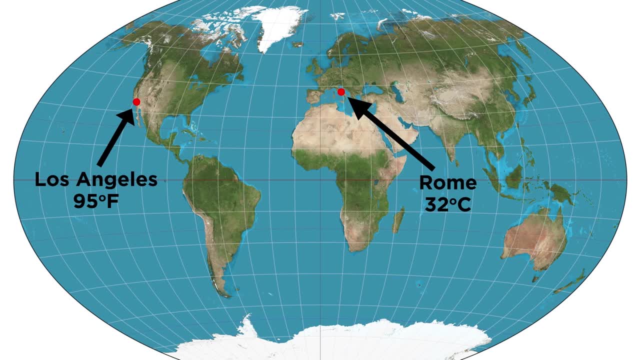 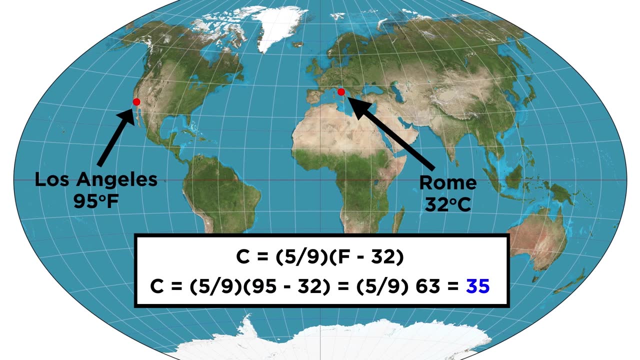 32 degrees Celsius in Rome. Where is it hotter? Well, let's take our Fahrenheit temperature, plug it in here and we get 35 degrees Celsius. Just to be thorough, It goes from 42 degrees Celsius into Fahrenheit as well. 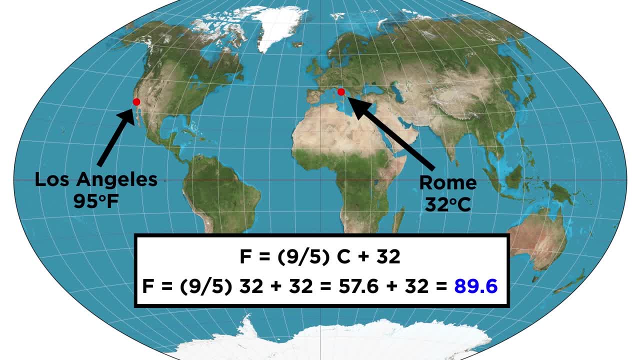 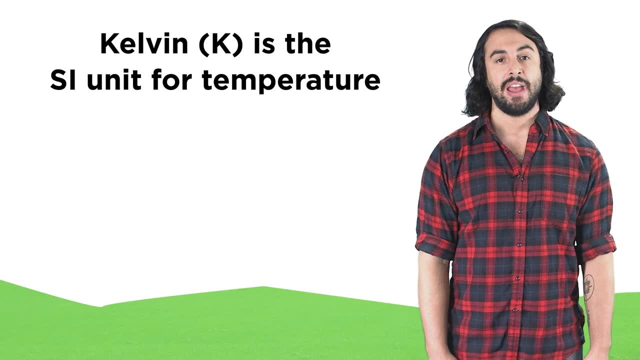 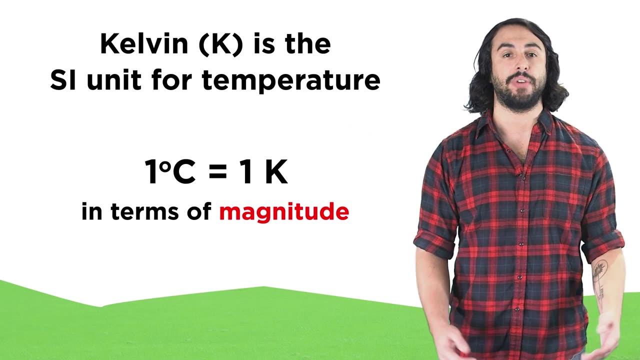 And we should get about 90. So it looks like California is the winner in this round. As we mentioned earlier, Kelvin is the SI unit for temperature and it is derived from the Celsius scale, in that one degree Celsius is precisely equal to one Kelvin. 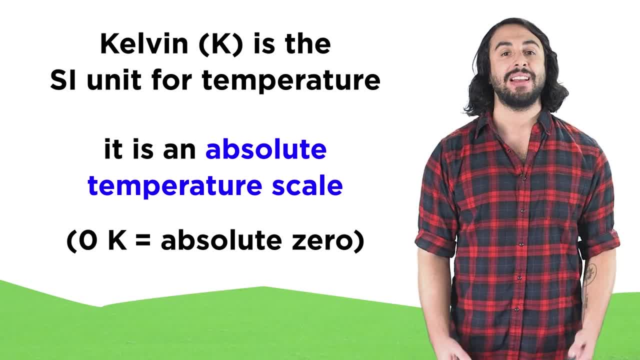 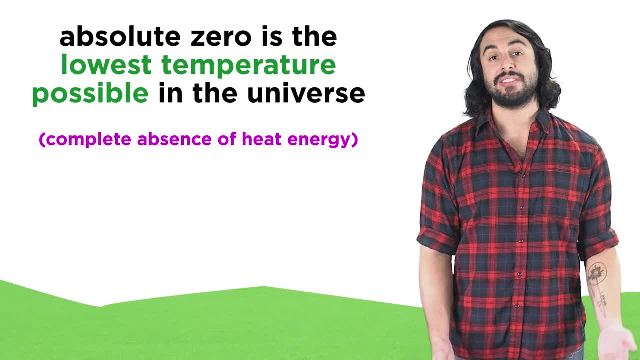 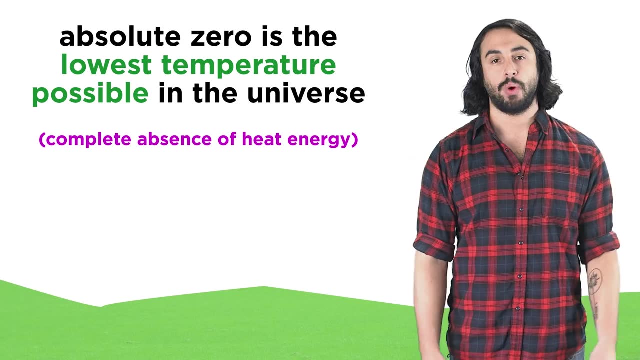 But Kelvin is an absolute temperature scale, meaning zero. Kelvin is absolute zero or the lowest temperature possible, Believe it or not. there is a lowest possible temperature because temperature is a measure of available heat energy. So if there is no heat energy whatsoever, you are left with absolute zero. 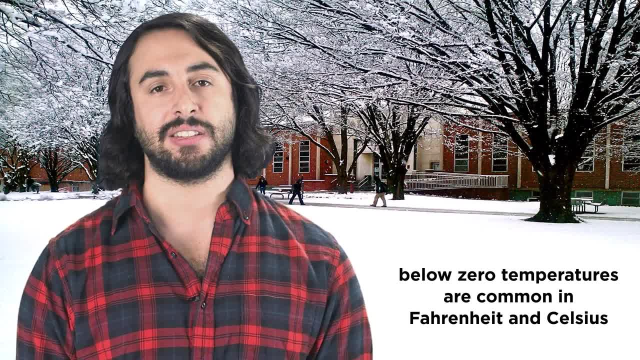 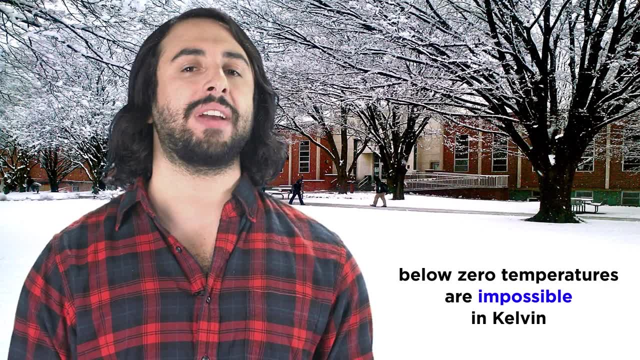 We are used to below zero temperatures in Fahrenheit and Celsius if it is very cold. But this is impossible in Kelvin, and for good reason, Because if we do calculations using certain equations and we plug in negative values or zero for temperature, 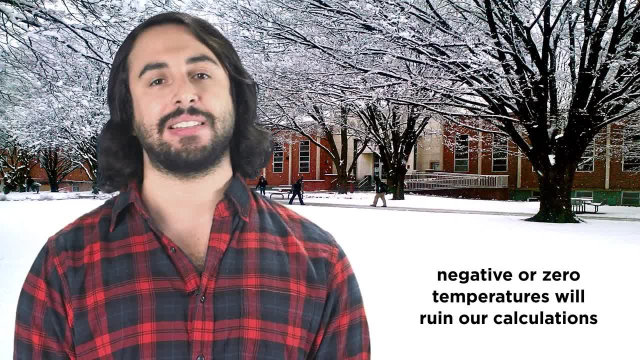 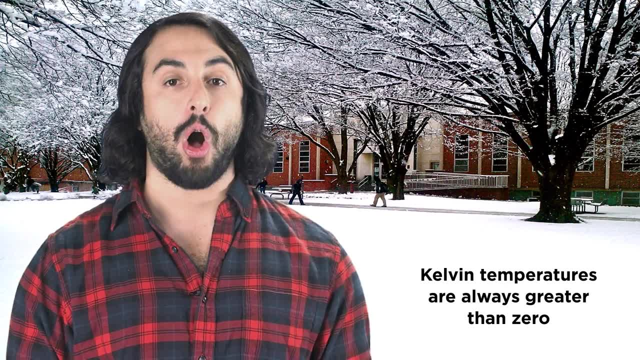 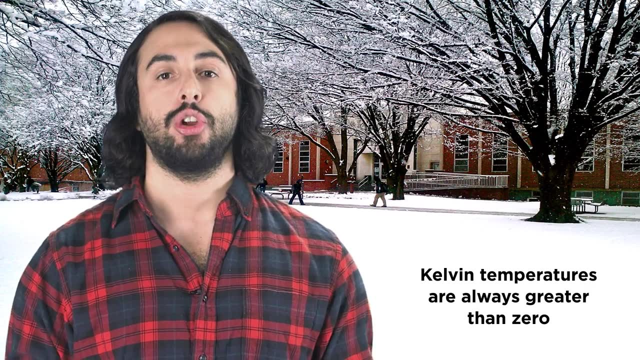 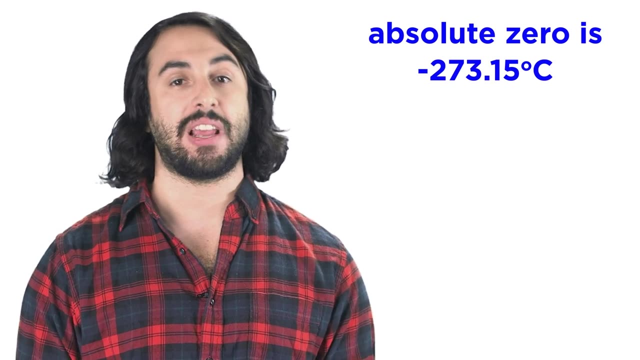 It will ruin our math, because it doesn't make sense to use negative values when discussing heat energy. We need a temperature scale that will always be positive, so that we can demonstrate the proportional change in a quantity due to temperature change. As it turns out, absolute zero is about negative 273 Celsius, which means we can use these.